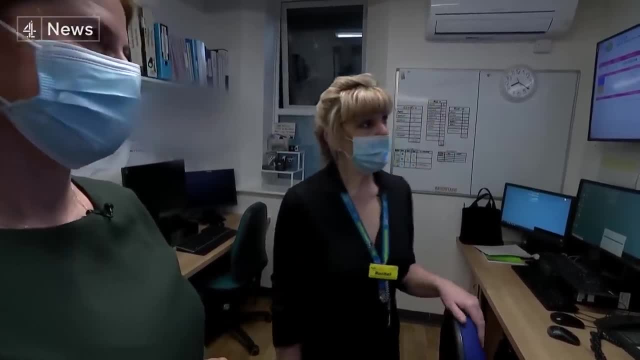 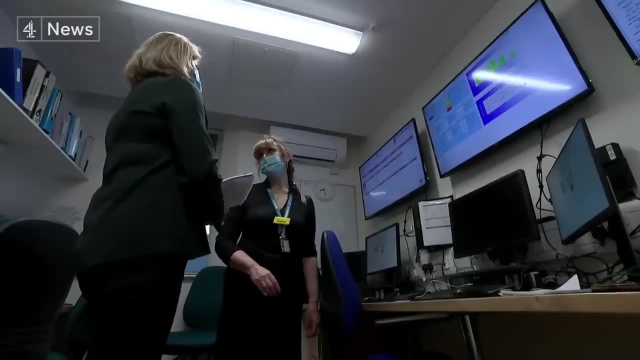 What does this mean for today? Is this busy? So yes, so this is busy. So we're minus 85 today, so we're in 37 escalation beds at the moment. This is the room with the data, and it was only. 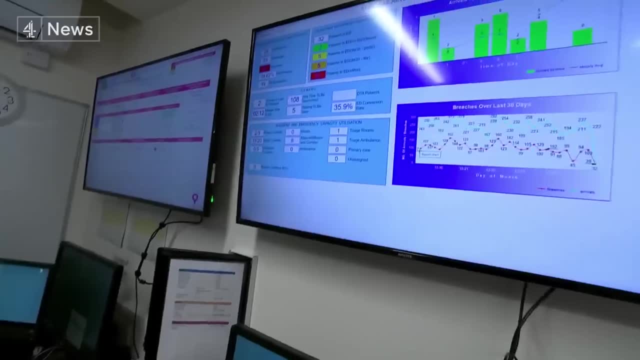 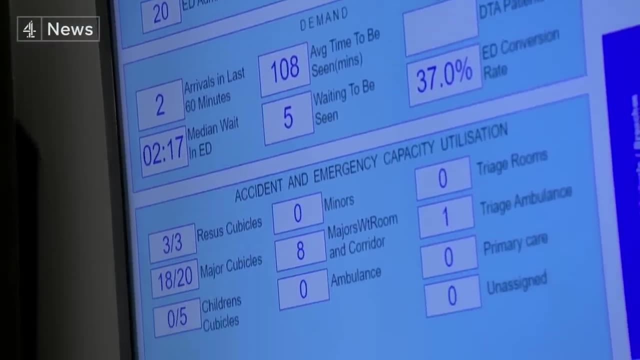 8.30 in the morning and they were overstretched. We can see we've got two out of three recessed cubicles, so we have a recessed cubicle available should we need it. We've got nothing currently in minors. We've got 19 out of 20 majors cubicles. 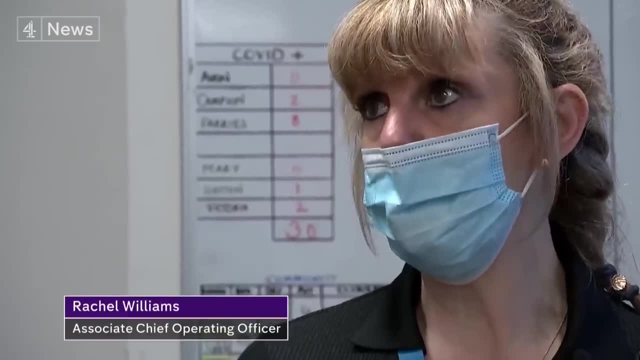 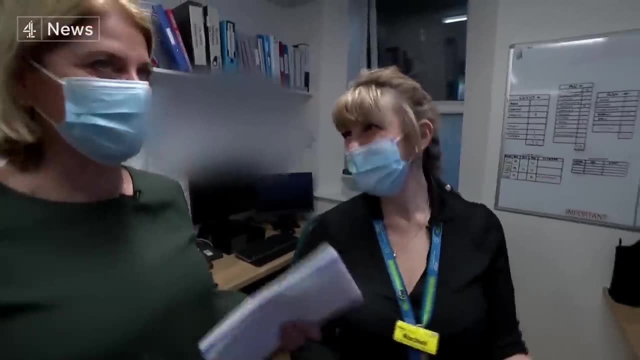 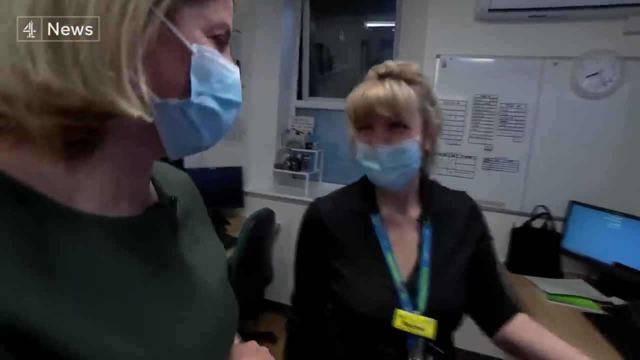 so we know that we're under pressure in majors already, which is where the ambulances tend to come, And we've got eight in our majors waiting room and our corridor. I don't even know how you keep it flowing. I feel exhausted for you And that's what. 25 past eight in the morning. 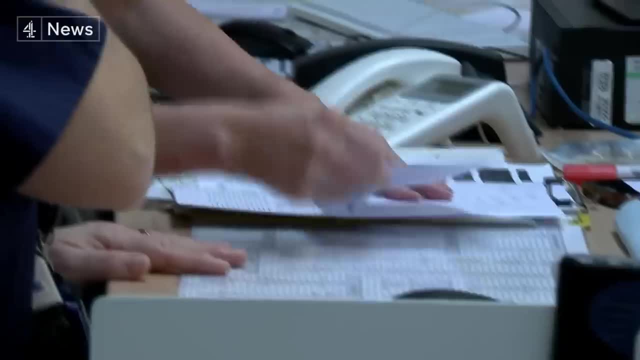 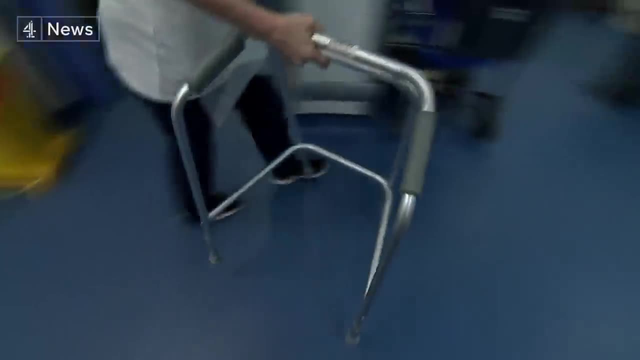 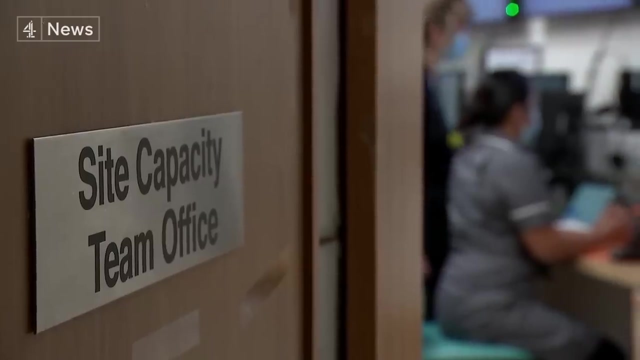 Nobody doubts the NHS is in crisis, a poly crisis across the service: Hospitals, yes, GPs, mental health, social care, The emergency department paints just one picture. Coming into our infection control prevention, we have a high rise numbers of our respiratory. 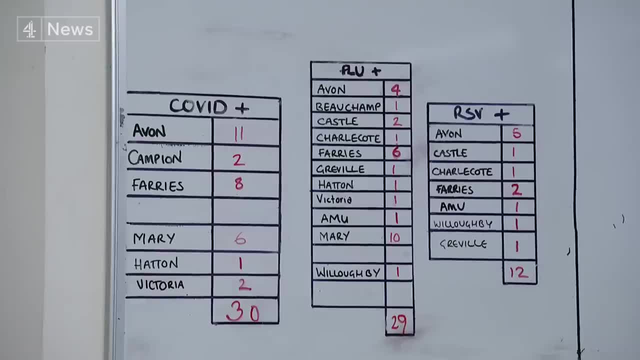 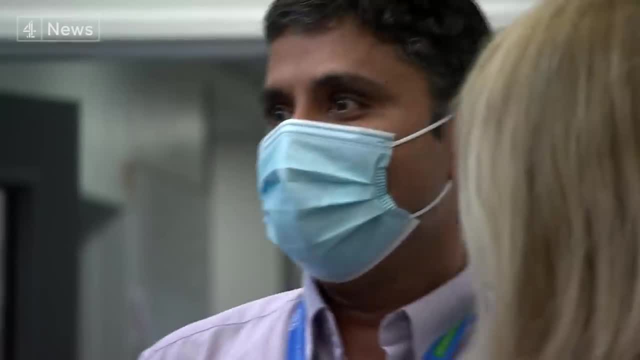 viruses And it isn't pretty: 71 who've tested positive for flu, COVID and those respiratory viruses. Have you ever known it? this bad Dad? I say every winter we keep saying this is the worst ever winter. so I suppose no is the. 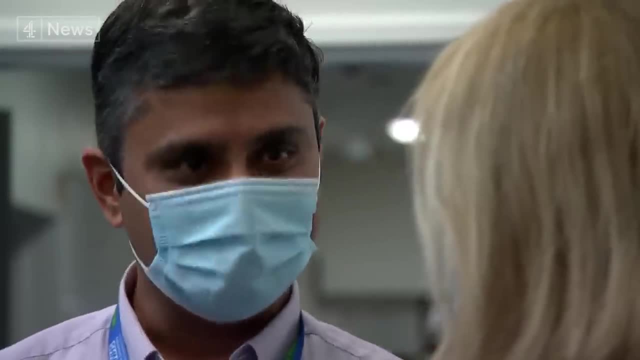 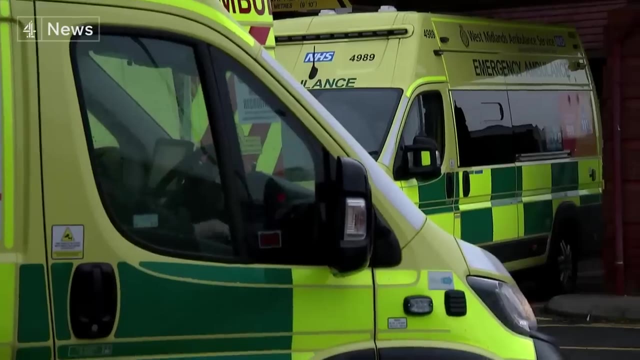 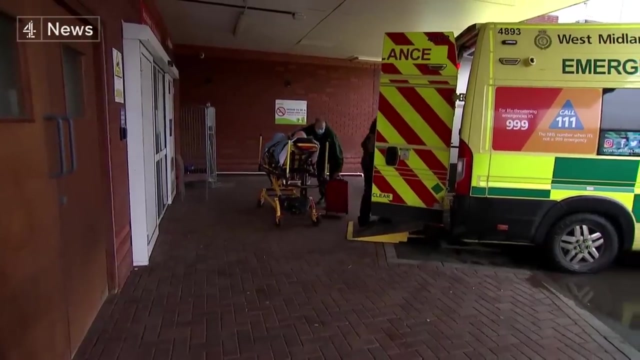 answer because of this twin and triple demix that we're going through. So it's bad, It is bad, It is bad. Figures from NHS England today indeed show that ambulance response times in December were the worst on record, And the proportion of patients seen within the four-hour target in A&E fell to a. 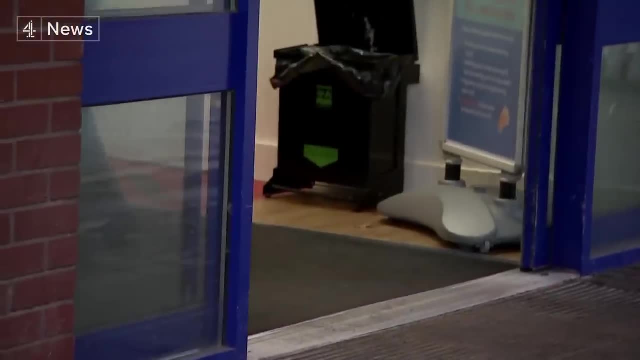 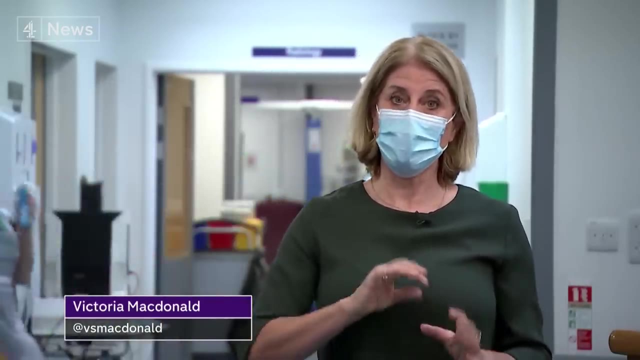 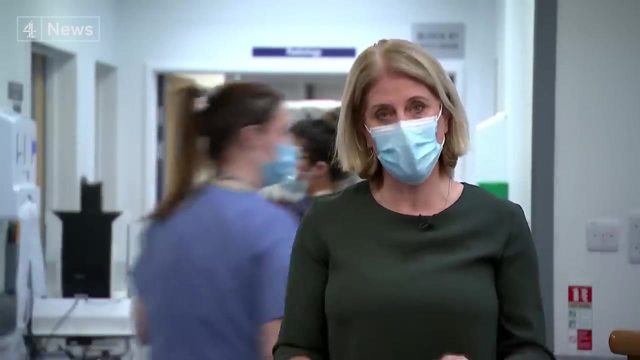 record low of 65% last month. Warwick Hospital has a number of different initiatives for keeping patients out of hospital or getting them back out into the community as quickly as possible, And yet it is still incredibly busy. The hospital is full And one person has just said to me frankly: 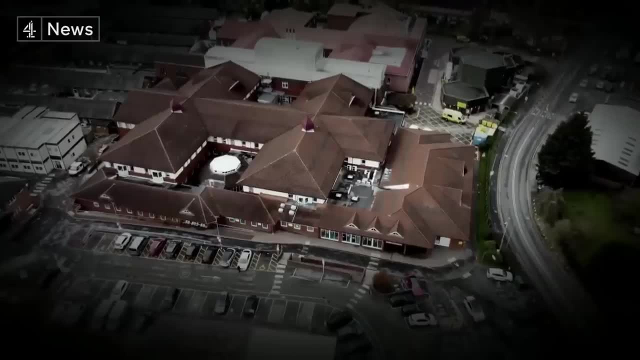 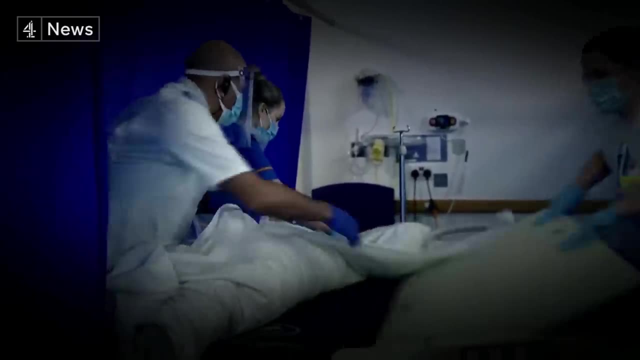 it's about managing a bad situation. Nearly two years ago, we filmed here 12 months into the pandemic and we spoke to Avon ward manager, Sarah Rawlings. It's emotional, It really is. It's been a tough 12 months. 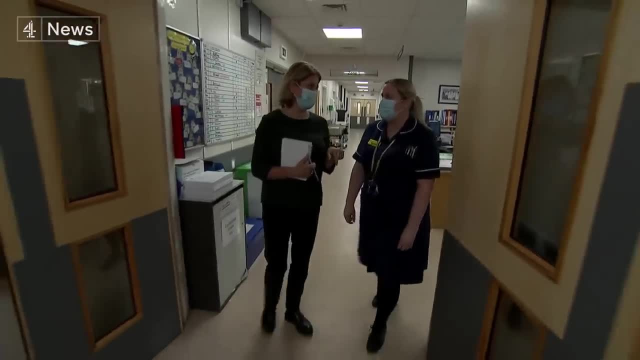 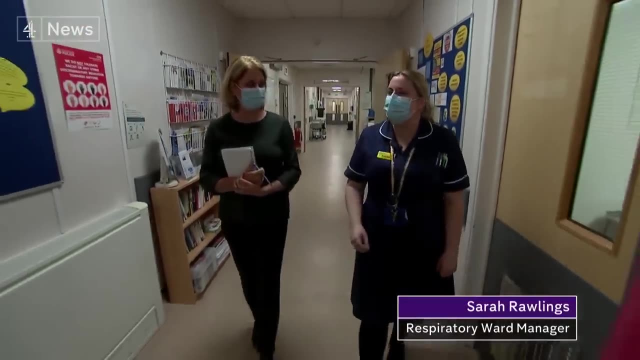 Sorry, I saw you two years ago. Two years ago, yes. So what's changed? A lot's changed, but then a lot is still the same. So we are still COVID, but we are also this winter. the impact that has changed is we now have all the other respiratory viruses. So 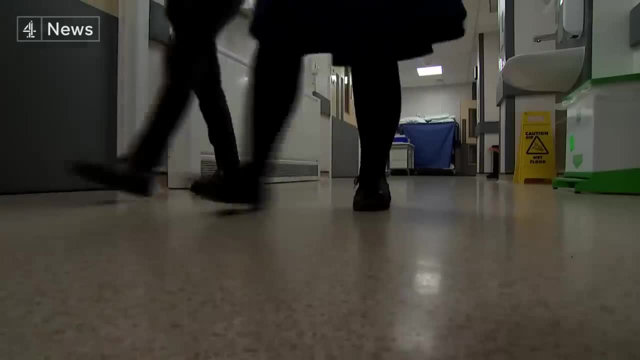 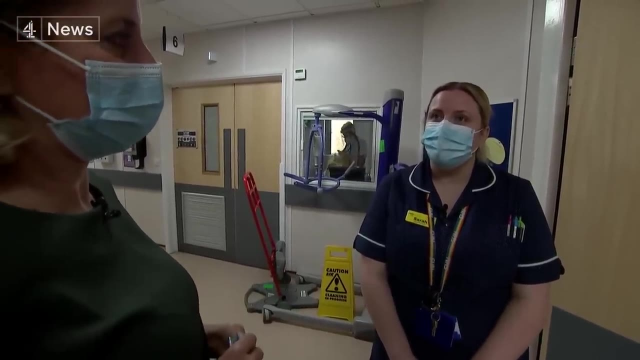 we're seeing a rise in flu A and RSV, and we have all those on the ward as well. There's been a lot of talk from the government about the NHS needing to be more productive. Could you be more productive? I don't think we could. 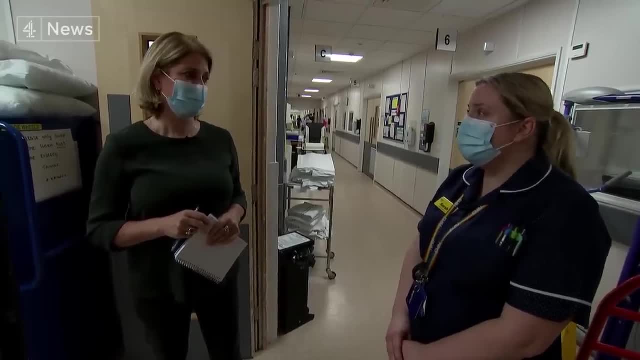 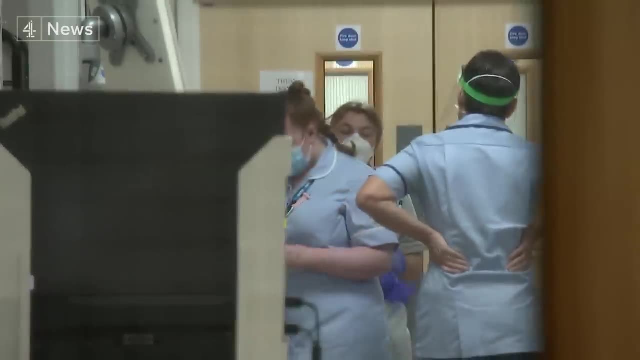 No, my team. we don't stop. We're busy, We're constantly on the go, We are constantly full to capacity, having to use extra capacity where we can. And here's the thing: This is a hospital awake to innovation, full of ideas for how to lessen the load. 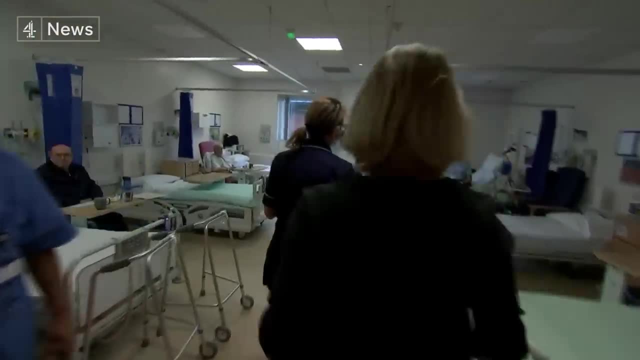 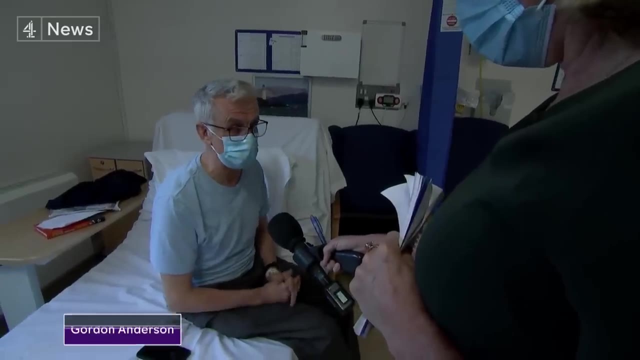 The medical day case unit was set up last July to avoid admissions, So this patient has come direct from the GP into MDC. I've come here because I've recently had a catheter fitted, I've got a urethra, I've got a urinary issue that's going to require a prostate procedure. 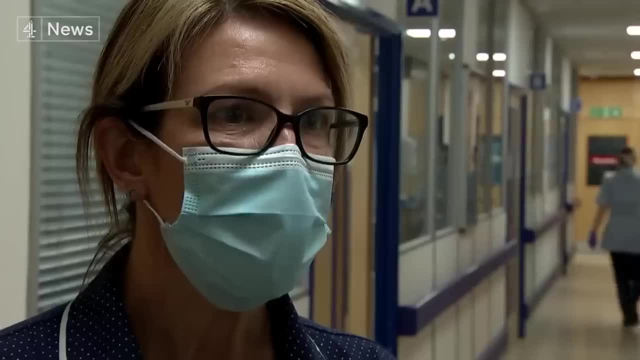 And what would have happened? normally He would have gone into ED and possibly been admitted. He wouldn't have been admitted, but he would have waited there for a very long time to be seen. He would have obviously not been priority to be seen in A&E. 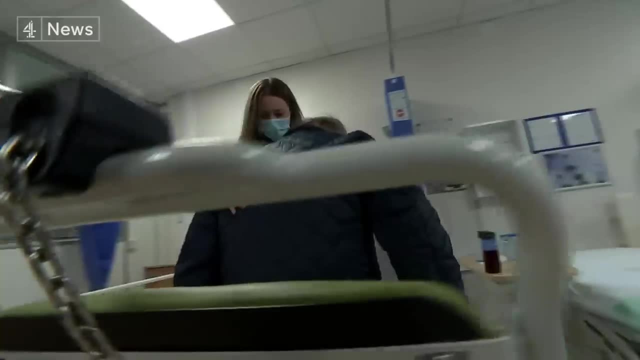 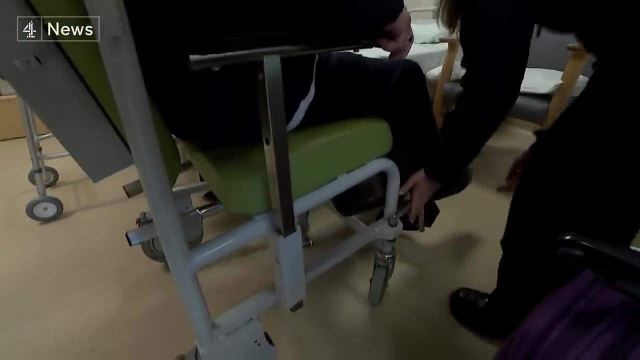 So he would have waited in a queue where there's more serious people that need to be seen. On average, 13,000 patients a day in England are in a hospital bed despite being medically fit. It's about 20% of inpatients at this hospital. 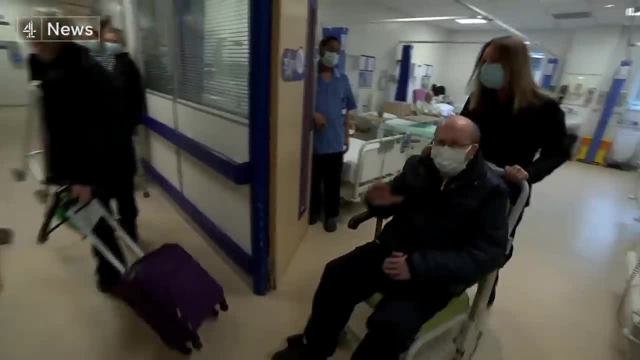 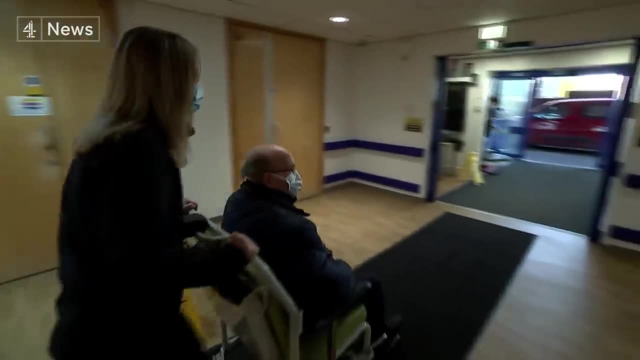 Are you ready to go home? But Michael Bradshaw is no longer a statistic. Bye, Michael. The Fire Brigade, Warwickshire Fire and Rescue to be specific, have set up a service to take patients home. It relieves the NHS. We get patients home a bit quicker. 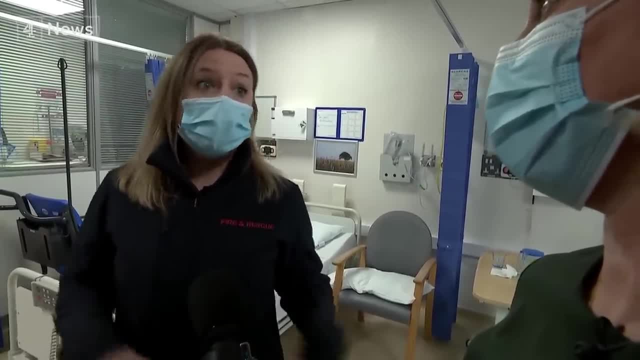 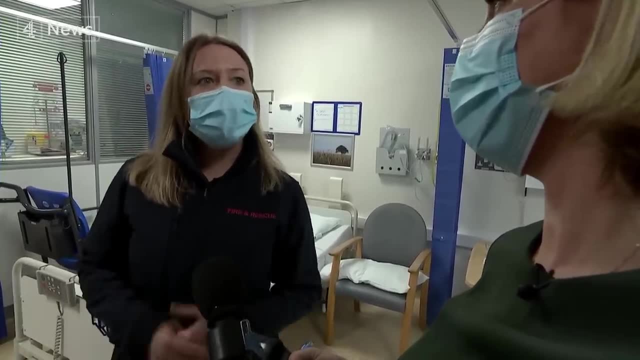 We only have to be at the hospital within one hour of the request coming through, So it saves patients waiting aimlessly and it clears beds for new patients coming in. And Dr Helen Dillon. Dr Dillon shows us a service which trains patients or their relatives. 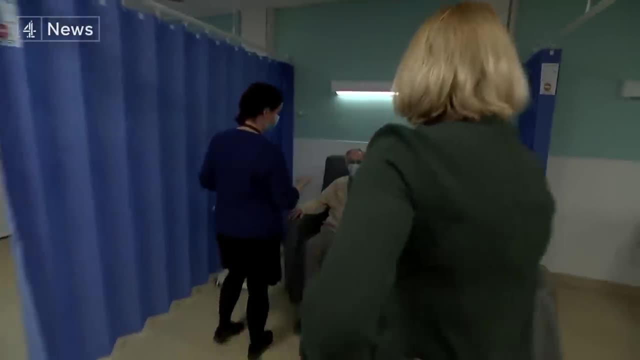 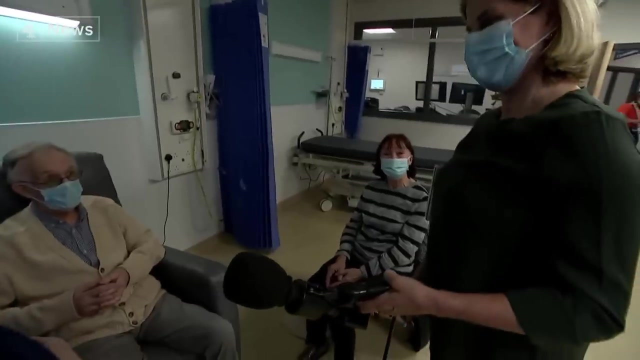 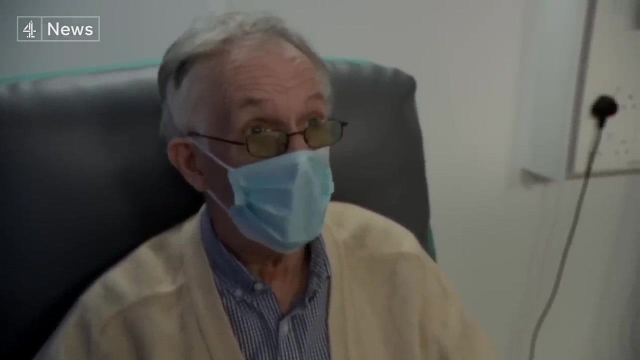 Hello, This is Mr Longstaff, to administer intravenous antibiotics in their own home. And this is Mrs Longstaff who's been delivering his antibiotics with our support and guidance. Why is it better? Because I've got the comfort of being in my own home, but a high level of treatment. 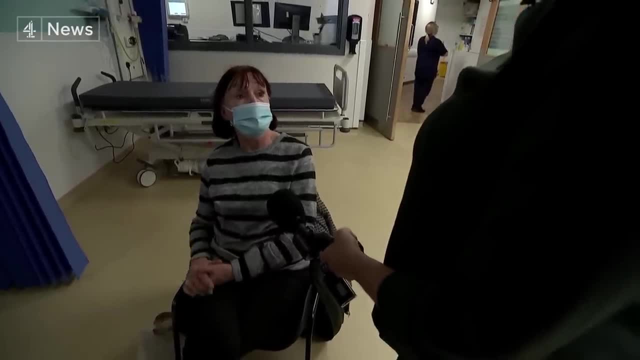 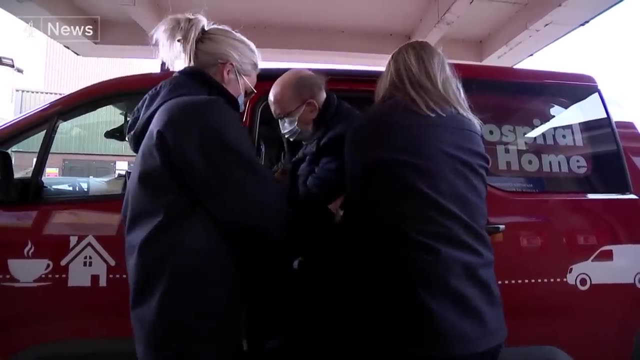 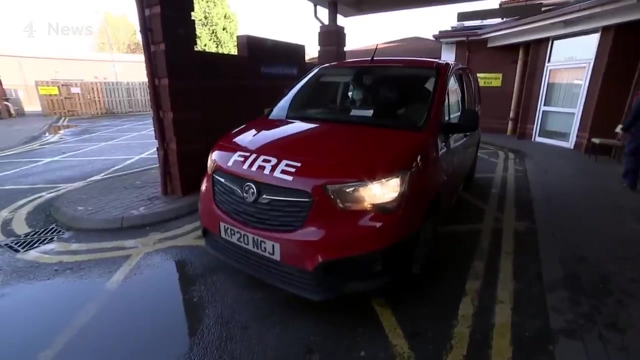 This sort of system. getting people home with treatment definitely is a plus. Putting together all the services, There were more than we can show. This was hundreds of patients being kept out of hospital beds And yet, for all the innovation, they were over-stretched. 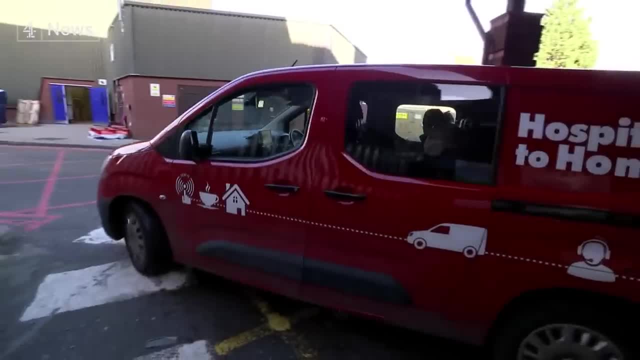 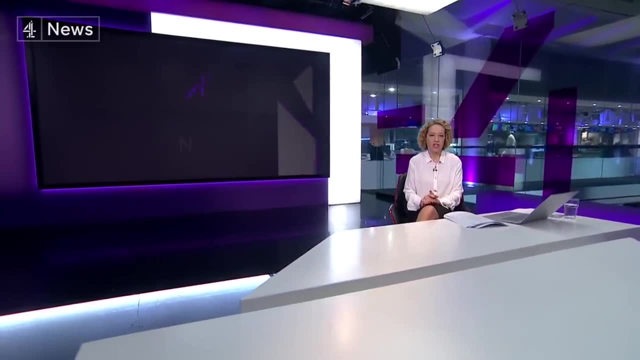 And there was still tomorrow, with many more sicker, frailer people to come. Well, NHS leaders say a staffing crisis is central to the pressure on the health service, A message they passed on to the Health Secretary, Steve Barclay, in talks this morning. 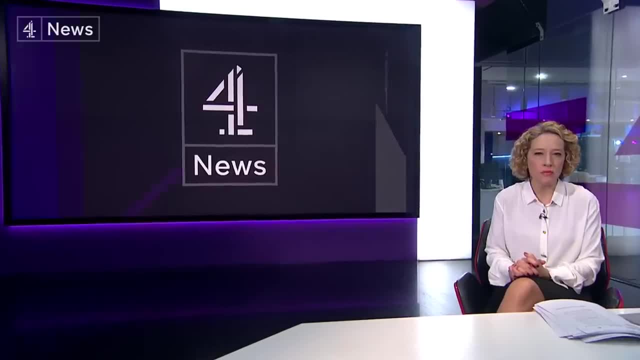 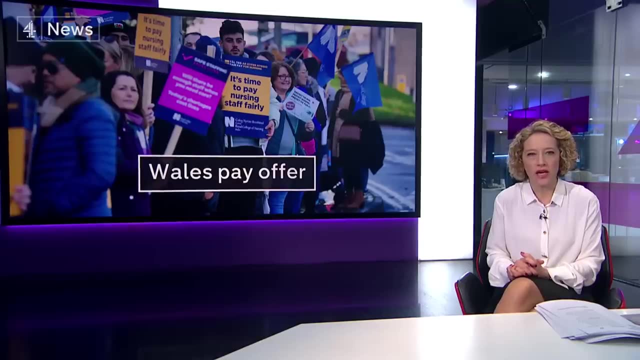 We'll be hearing more about that in a moment, But first the government in Wales has also been meeting health unions in a bid to avert strikes by nurses and ambulance workers. Its offer of a one-off payment hasn't gone down. well, Let's get more from our Home Affairs correspondent, Andy Davies. 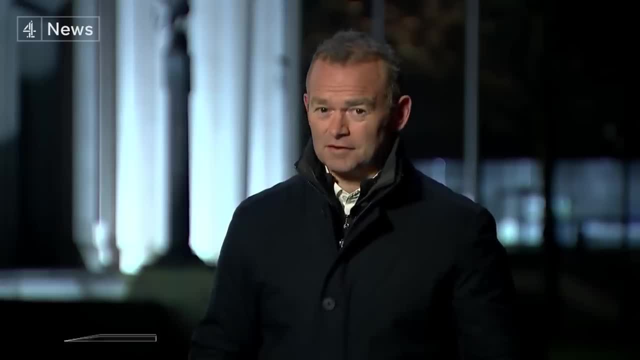 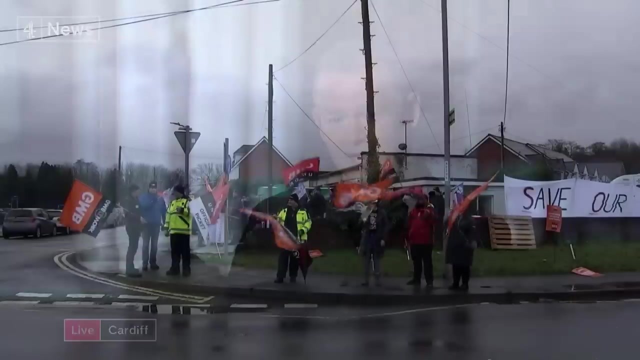 Andy, The fact that this meeting happened today some may see as progress, But if anyone had been hoping that it could yield a seismic moment in terms of resolving the strikes issue in Wales, well, it didn't get anywhere near that. It comes after another strike yesterday. 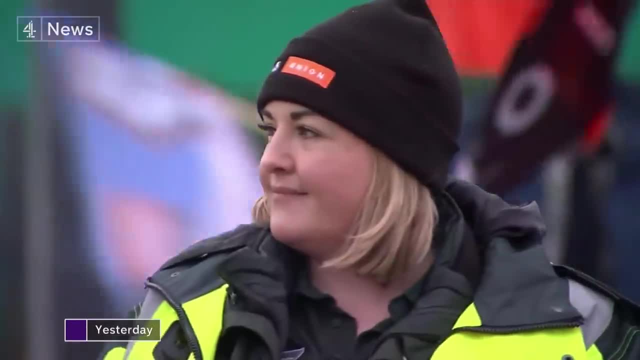 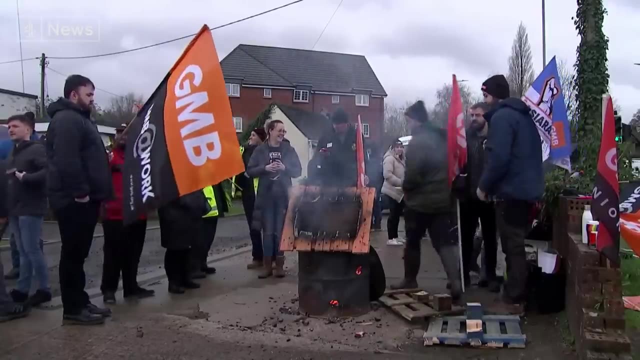 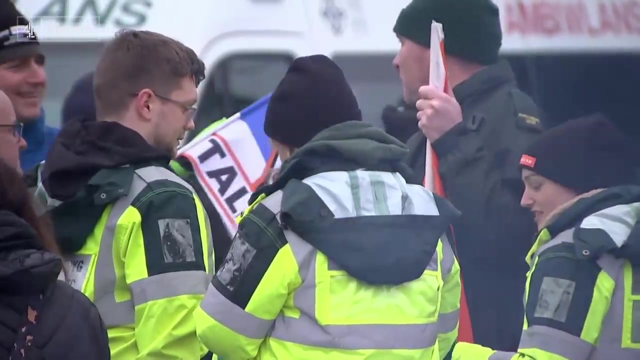 By ambulance workers in Wales, with more to come involving midwives and physiotherapists, And what the Welsh Government has been offering here is an overall sum of money to be used as a one-off payment. None of those involved in today's talks would disclose how much money was on the table. 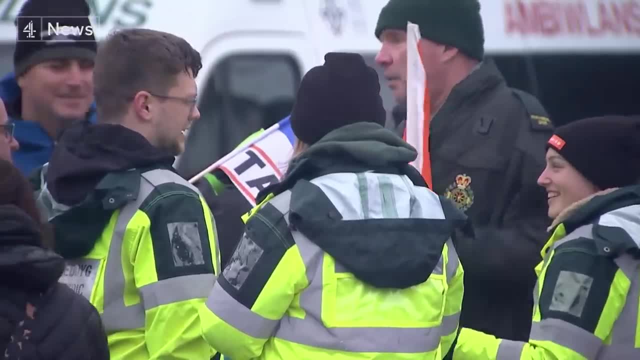 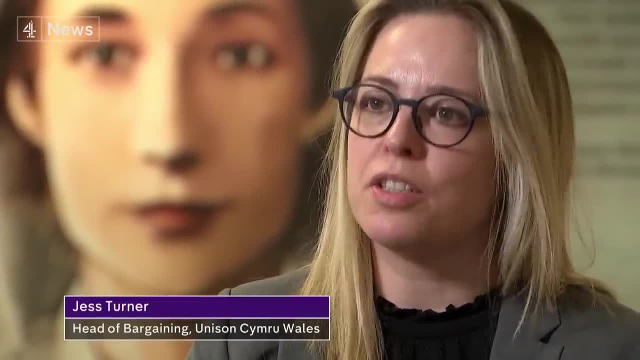 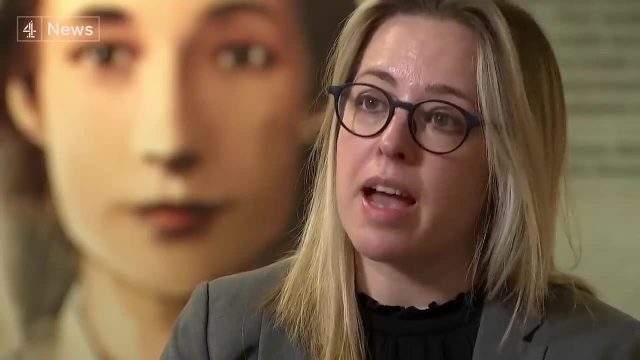 They pitched this as that they want to do this. They said they wanted to do something for health workers, But the money just simply isn't there. So they said they've looked at budgets and where there have been underspends and areas where they can potentially claw back some money. 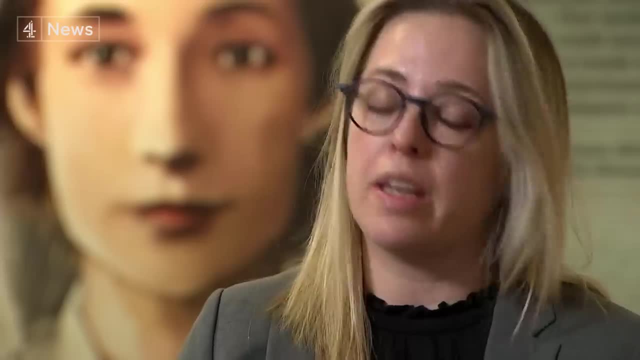 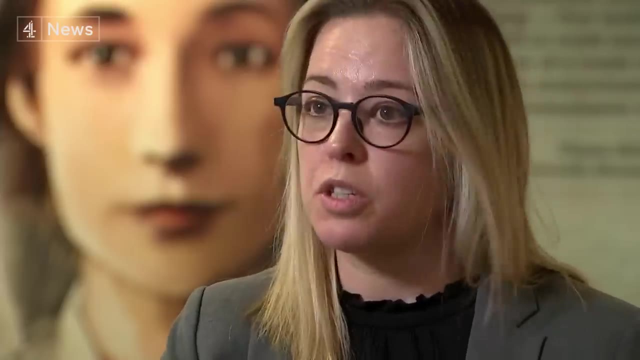 And they've put together a package that they say is basically all that they can afford. The importance, How much is that? I can't tell you at this stage because we're very much still in negotiations. So, in the spirit of those negotiations, I'm not going to share the figure. 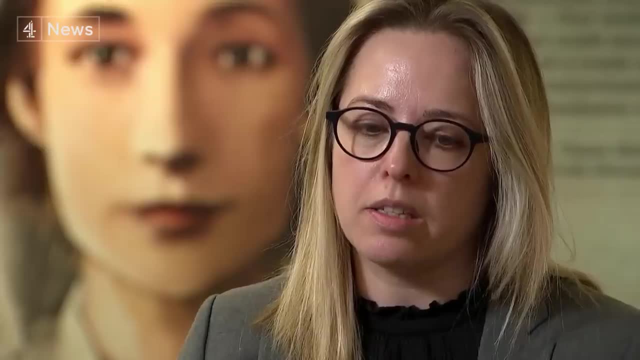 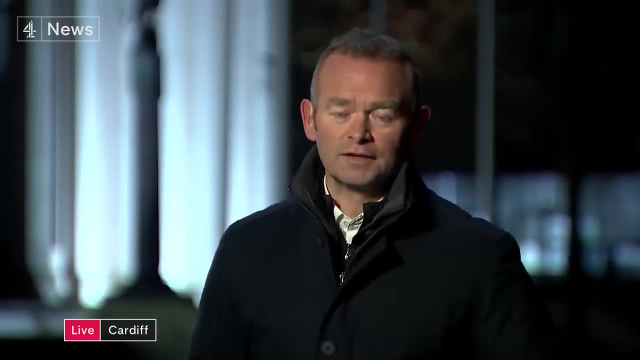 But what I can tell you is that the amount is unconsolidated, In other words, it's not permanent, it's a one-off. And as welcome as these talks are, she went on to say, that creates a problem because it is not what the unions have been calling for. which is a much improved year-on-year pay rise, which the Welsh government, in turn, claims that it can't offer without further funding from Westminster to Wales. Well so, Andy, what are the next steps then? Well, the unions say they will get together to discuss this. 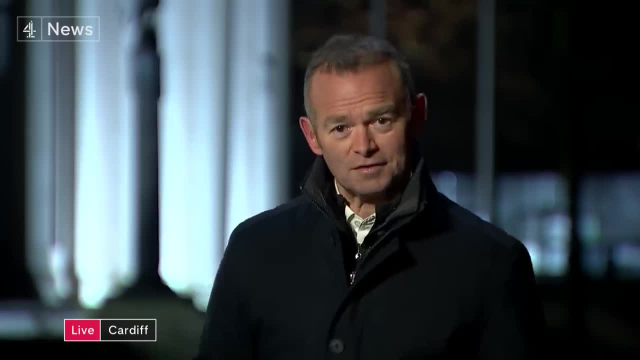 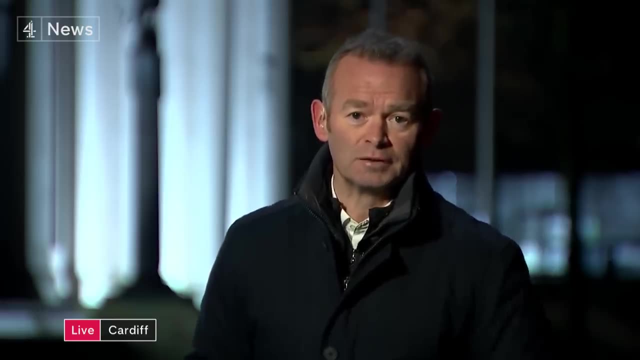 but that could be pretty brief, because some of the unions involved today- certainly those who've been on strike- have given this very short shrift indeed. Have a listen now to Helen Wiley from the Royal College of Nursing, who came out and afterwards said that the Welsh government 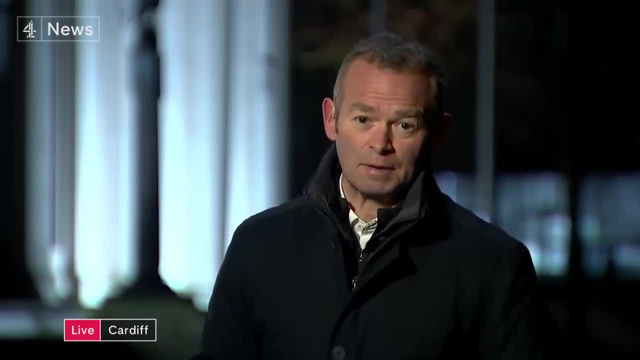 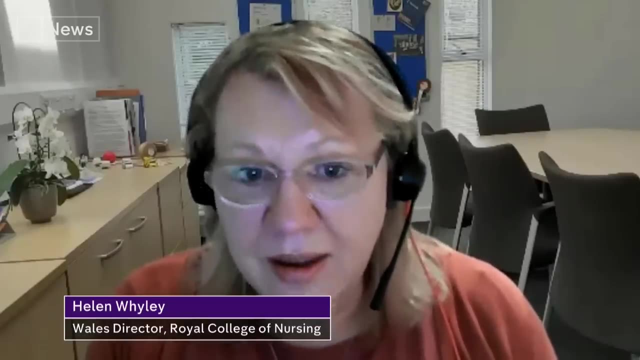 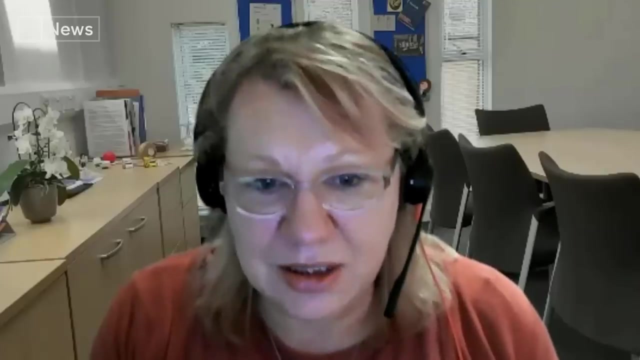 had not been negotiating seriously on NHS pay. This conversation today, whilst it's welcomed to be round the table talking, it falls very far short of any resolution of our dispute. So unless the Welsh government can change that approach urgently, we will be in a position where we will be considering 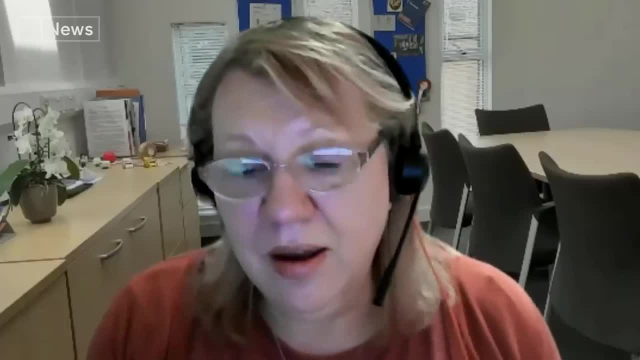 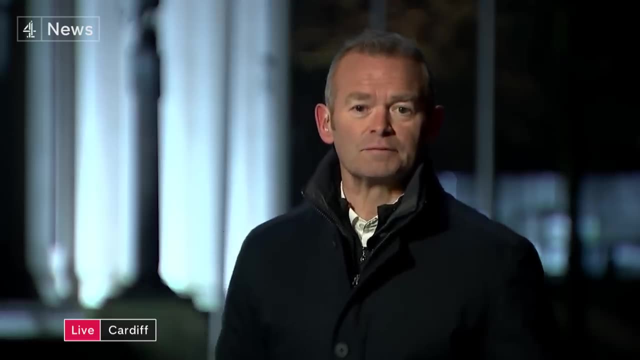 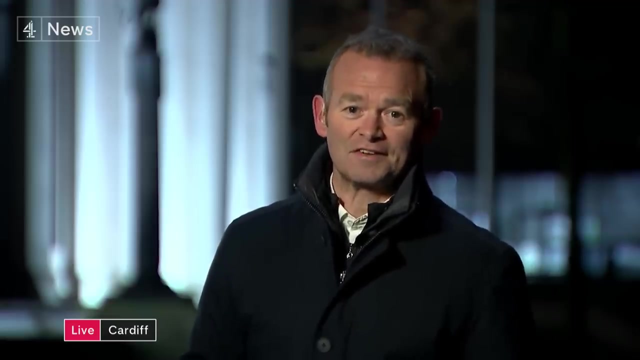 potentially further strike action and we will make an announcement about that imminently. Well, the Welsh Health Minister later said that she hoped these discussions can continue And from the soundings we got well, it's likely they will continue, but it's also very likely at this stage. 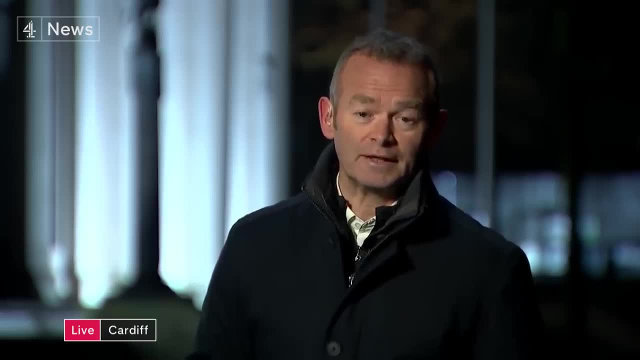 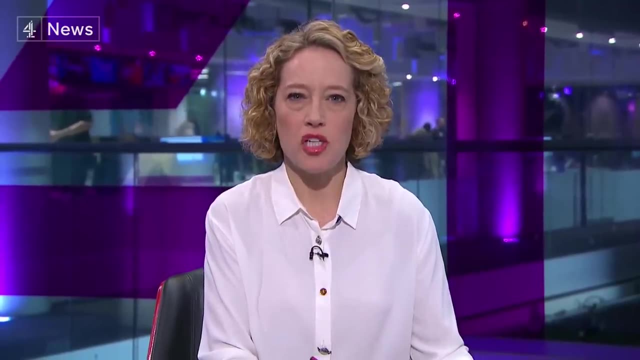 that they will do so against the backdrop of continuing industrial action. Andy, thanks very much. Well, earlier I spoke to Professor Philip Bownfield, who chairs the British Medical Association's UK Council and was at the talks with the Health Secretary today. 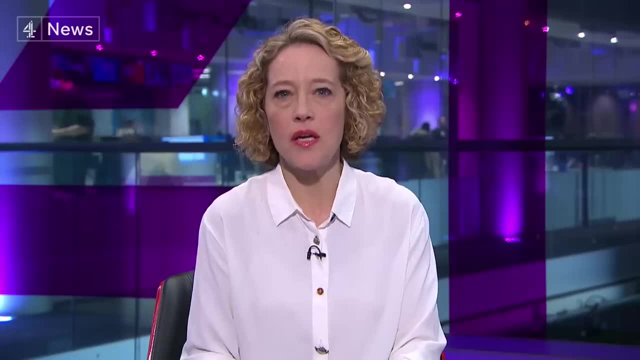 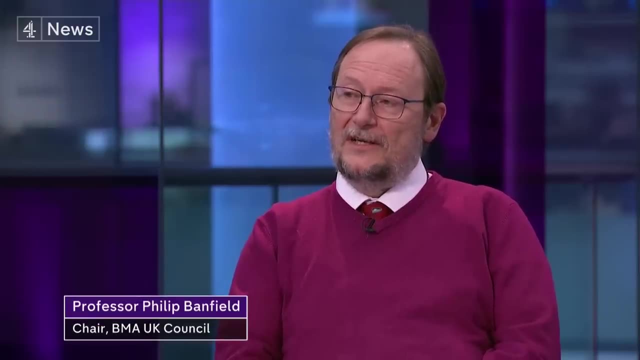 I began by asking whether, in his long career in medicine, he's known anything like the pressures we're seeing in the NHS today. Well, I've been in medicine for over 35 years and it's never been this bad. We've talked about winter pressures every year. 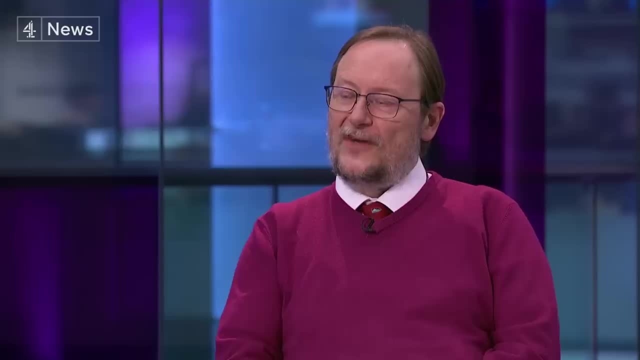 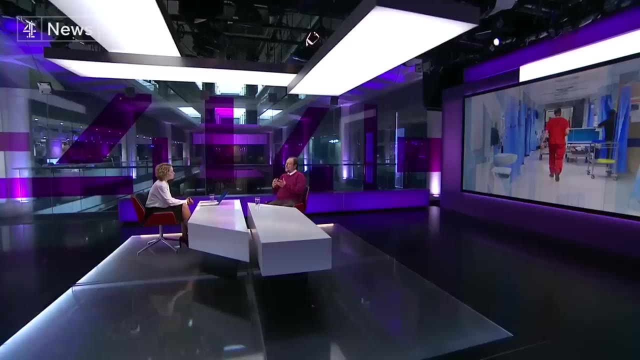 saying that they're getting worse. We're seeing winter pressures into summer and we're seeing the pandemic being blamed for the current state, But really it is year upon year of underinvestment. The public's experience at the moment is of an NHS. 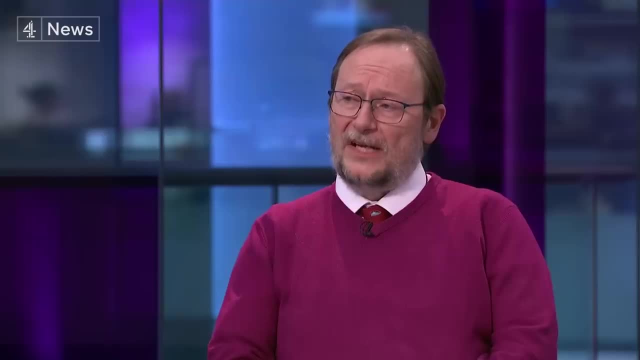 that is either near to or has actually collapsed in places. Has it actually collapsed already? Yes, Has it turned? Well, you know it has. We're seeing doctors and nurses with burnout, the moral injury from not being able to treat patients. 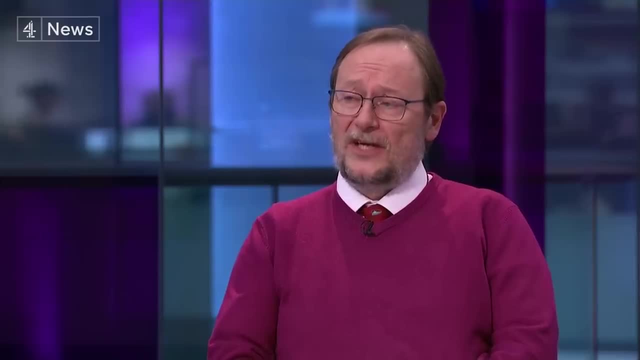 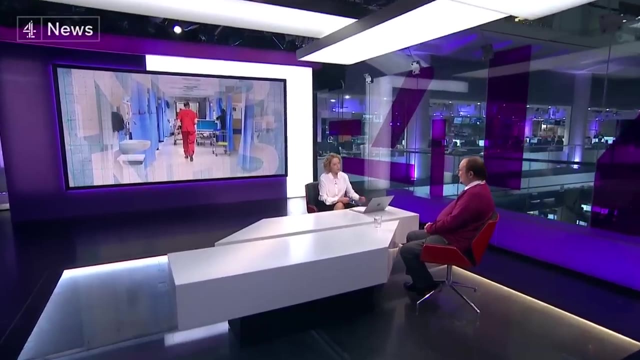 We're seeing patients saying: please don't send me to hospital because I don't want to be on a trolley for 24 hours. But you're going to make that situation worse if junior doctors go on strike, aren't you? Well, I mean, junior doctors feel that they've got no option. 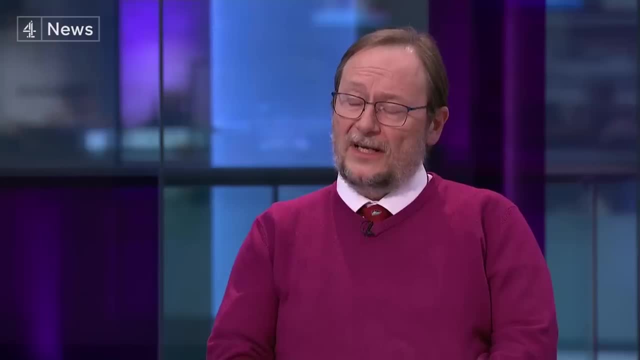 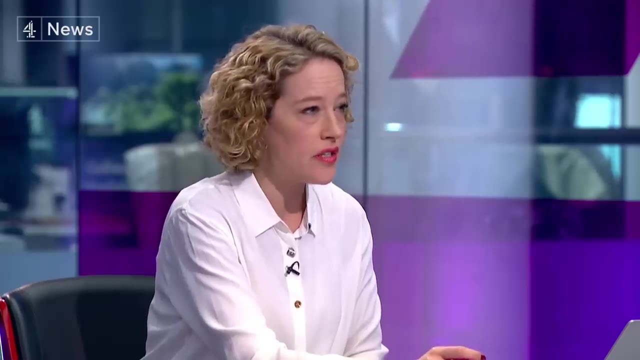 but to take industrial action because the government, frankly, isn't listening to their plight. You had talks with the health secretary today. Have you got any hope that you can avert this strike? The initial meeting with the secretary of state today: 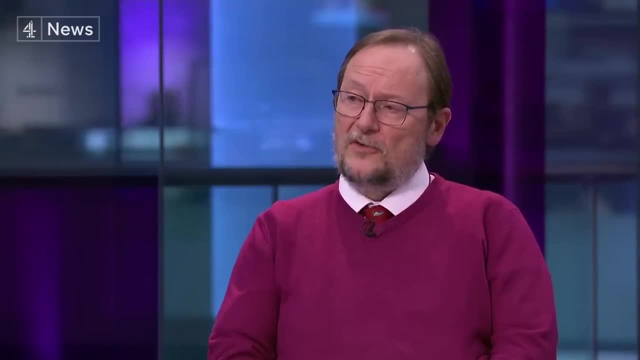 was positive. He listened, We were able to set out our stall, We were able to say that really there is no solving the problem with junior doctors unless the government considers full pay, restoration And reform of the doctors and dentists review body. 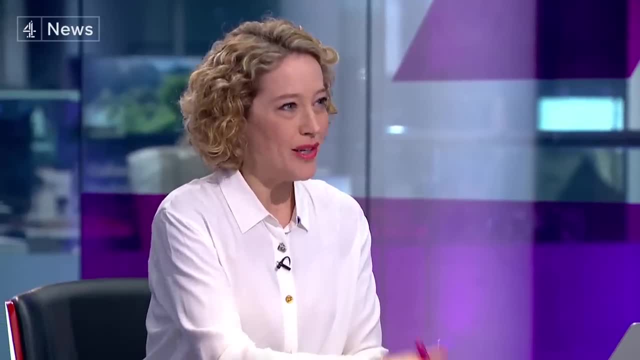 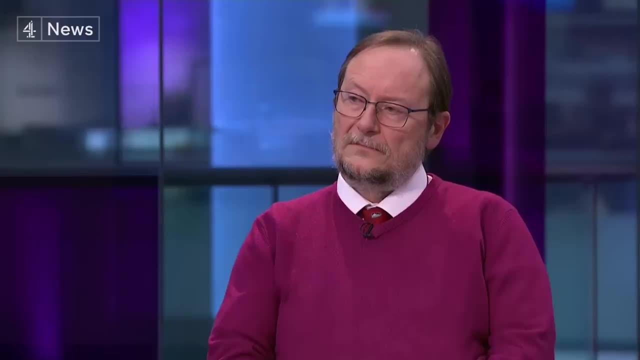 You've talked about years of underinvestment by the government, and you know we ask ministers all the time about that. But would you accept that members of your union also have some responsibility to participate in reform of the NHS? Yes, I don't think anyone thinks that the NHS can continue as it is. 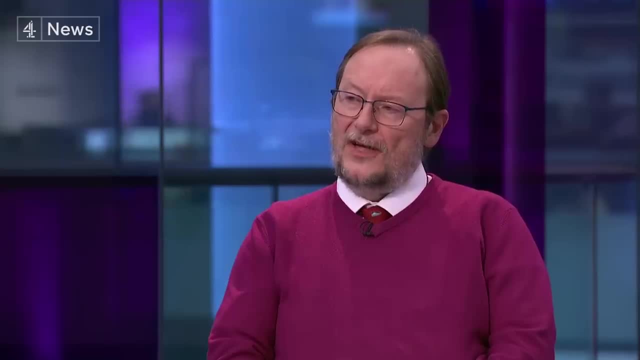 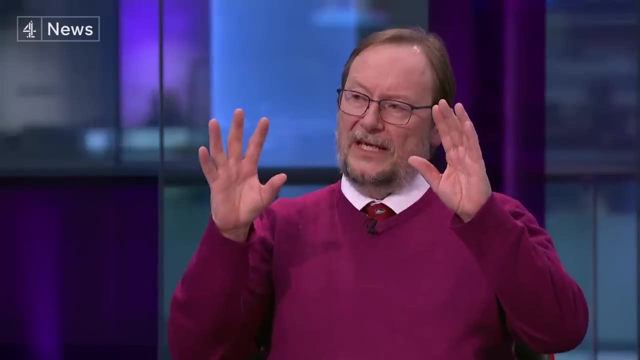 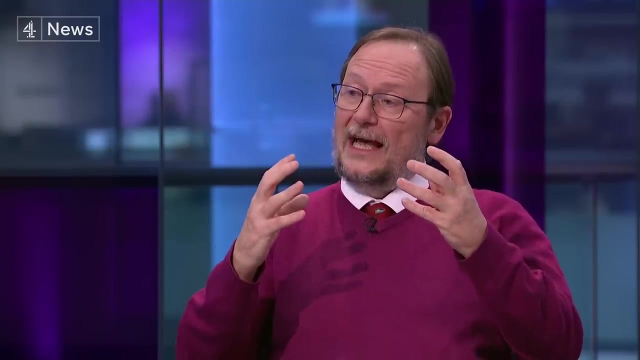 But if you're going to have redesign of a health service or meet the expectations of a the public, if you're going to go from Health Service A to Health Service B, then there is a transition both in terms of the service model and also the funding. 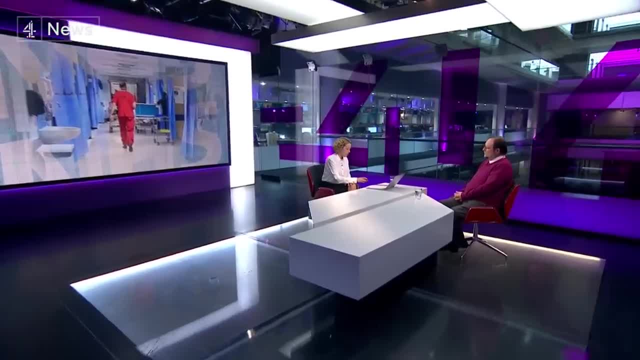 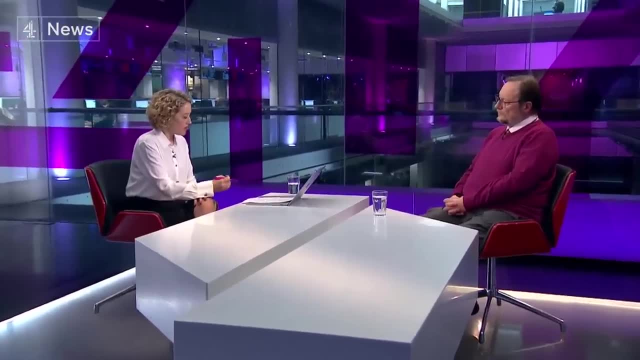 But you know, the IFS did a report saying that there'd be more funding, more staff, but the NHS was treating fewer patients. And when Wes Streeting, the shadow health secretary, took you to task on some of these things, 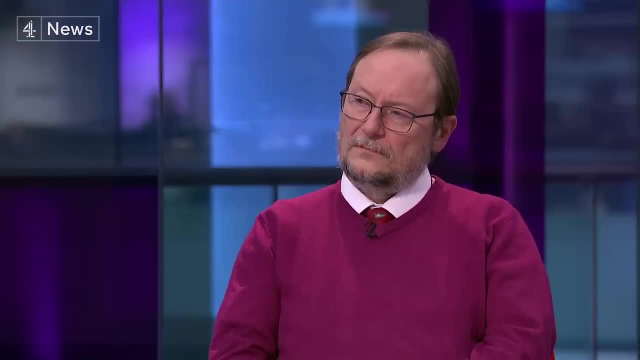 he says he was treated as some sort of heretic by the BMA. Well, I think I've met with Wes Streeting this week, so we have- You've built some bridges. ironed out some of the comments that he's made.